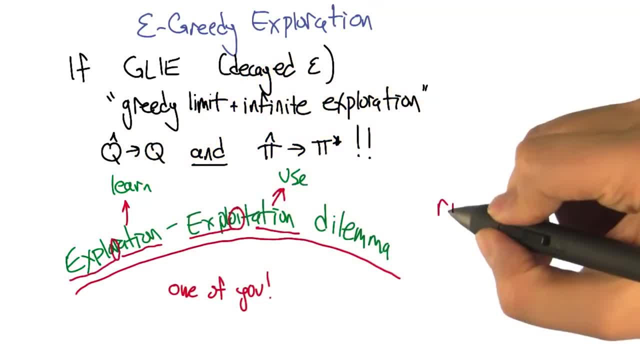 Oh, that's interesting too. Huh, So if you take an R and turn it into an it, you move from exploration to exploitation. I feel like an entire political movement could be founded on that. I'm not sure exactly what it would be. 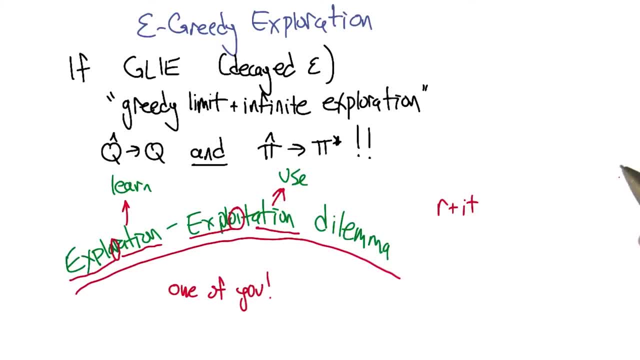 Maybe I'll work on that before our next lesson. So I have an algorithm there's. there's a standard lemma, Mm-hm In reinforcement learning theory called the Exploration Exploitation Dilemma. Sorry, no lemma, the other kind of lemma. 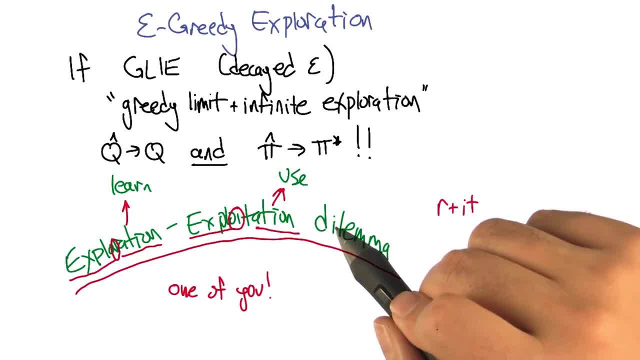 The Exploration, Exploitation Lemma, which has to do with taking actions that are either exploring or exploiting. But I have one where you actually do teaching, You can actually. each time you take an action, it's either going to teach the agent something it's going to explore or exploit. 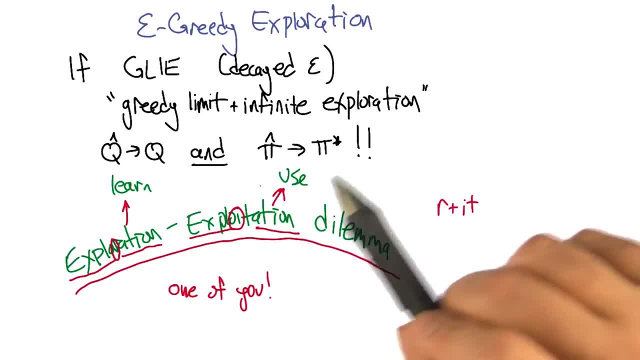 So I call that Exploration Exploitation or Explore, Exploitation, Exploit, Explain, Oh nice. But you could have called it the Exploration Exploitation Dilemma, because you used a lemma and di means two sometimes and you do the two things. 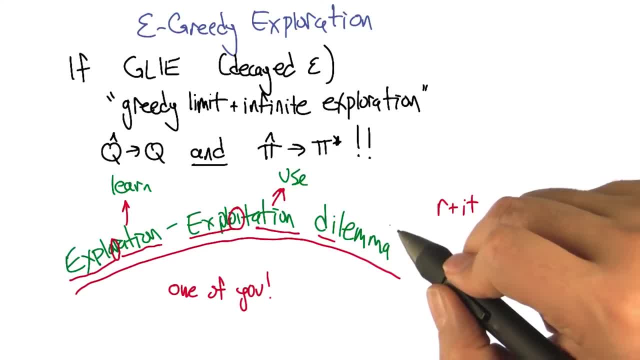 Well, in fact, dilemma does literally mean two. It's a choice between two things, Right, so it's a dilemma. Nice, It's a lemma about two things, All right. so there's, it turns out there's a lot of other approaches to. 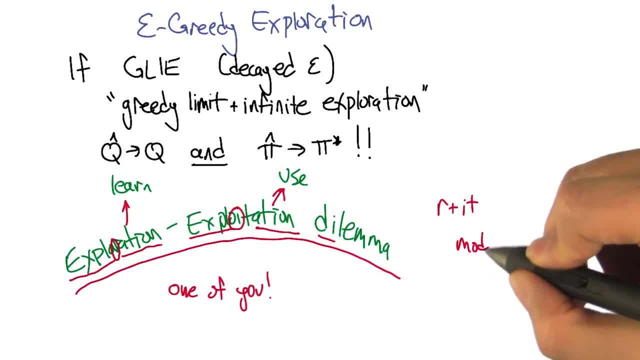 exploration, exploitation and some of them in the, in the model base setting. you can do a lot more with it, a lot more powerful things with it, because you actually can keep track of what you've learned effectively in the environment and what you haven't. 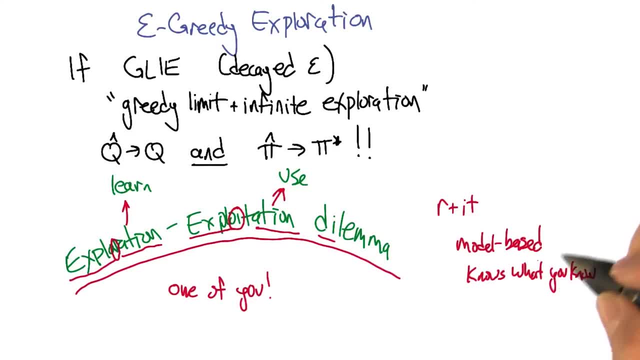 So the algorithm can actually know what it knows Mm-hm, And can use that information to explore things that it doesn't know and exploit things that it does know. Q-learning doesn't really have that distinction. It's a much harder thing to do. 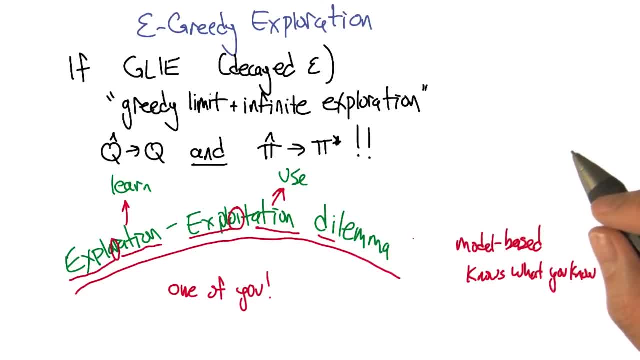 Hm. So so that's what I wanted to tell you in terms of, you know, thinking about exploration, exploitation. Does that make sense to you? It does make sense to me. I think the main point I got out of this, or a main point I got out of this- 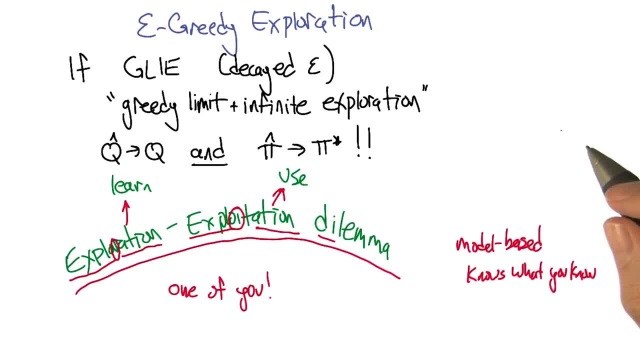 other than our incredible ability to get caught up in letters and coincidences of spelling, is that the exploration- exploitation dilemma really is a dilemma. It's like the fundamental trade off in reinforcement learning: You have to exploit because you have to use what you've got. but 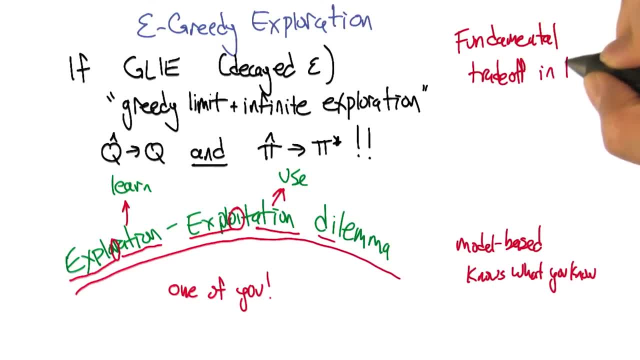 you have to learn, or otherwise you might not be able to exploit profitably. So you have to always trade off between these things, and if you don't, you're bound to either learn nothing or to get caught in local minimum. I couldn't agree with you more.